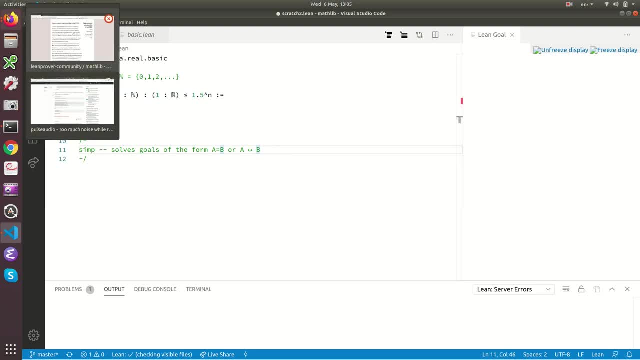 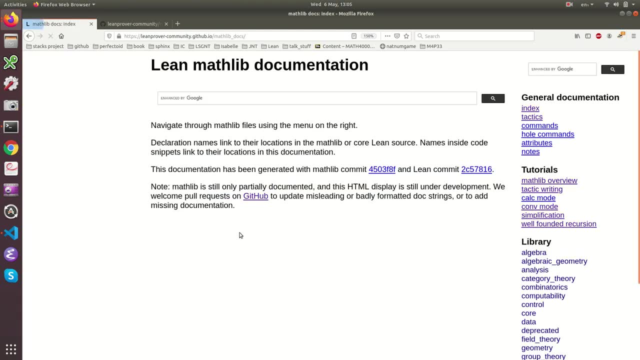 Another tactic which I should say that there's a lot of tactics. you see, if we go to the LeanProver community website here, then click on the API documentation then and then click on the tactics, you can see that there's a huge number of tactics here and one thing that one can do is to start. 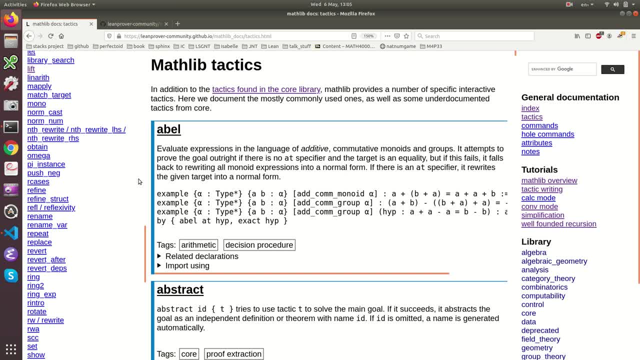 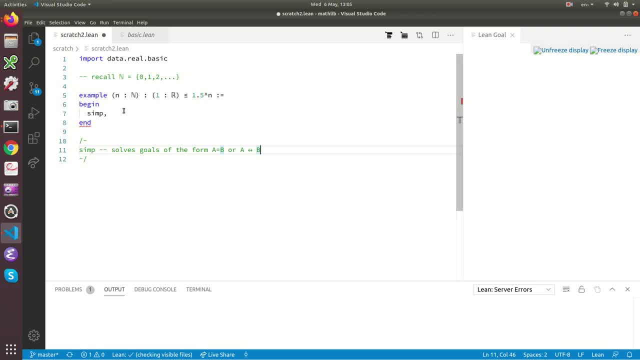 plowing through the tactics and seeing if one can find one which will solve this goal, But in fact that's somehow doomed to failure, because no tactic, no one tactic, will solve this goal, for reasons which will perhaps become clear in a minute. So the next thing is: this is an inequality and it 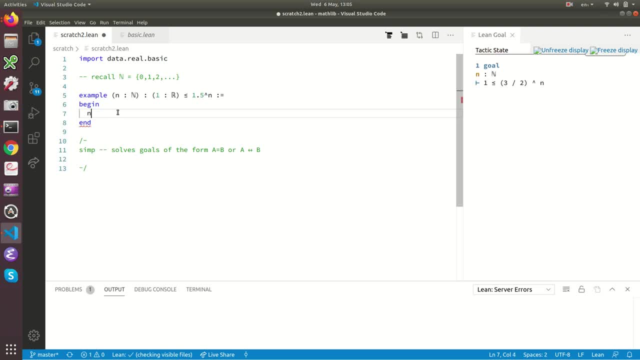 involves numbers, and so you could try. you could try normnum, see if that will solve it, and normnum will fail to solve it. It's done something. it's, I guess it doesn't. it's done the same as what simp did. it's changed one point five to the n, to three to the n, over two to the n, But unfortunately 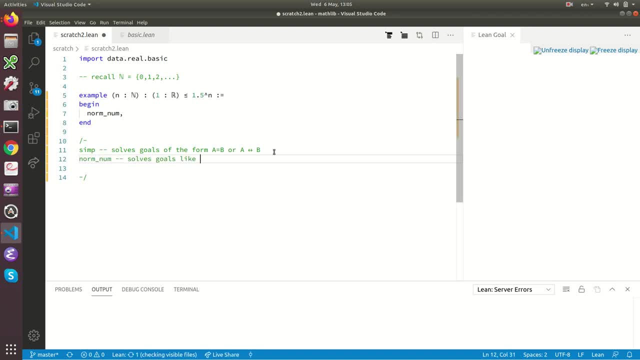 normnum. what does it do? it solves goals like kind of 1.5 is less than 1.7. normnum would certainly solve that goal, goals with numbers And this. you see, this isn't a number here, it's got some variable involved here. so normnum won't solve that goal. So the next thing you might want to try is: 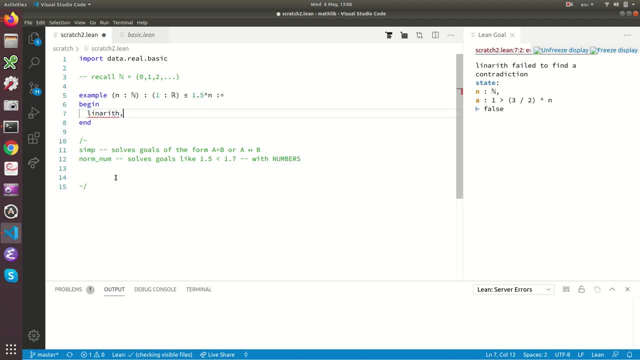 linearith, that will also fail, I would imagine. yes, linearith has failed because it solves linear inequalities. This one isn't linear, this has a power n in. And so now we're getting desperate. we're thinking: well, there's this tactic library search, which searches through the entire Lean's entire maths. 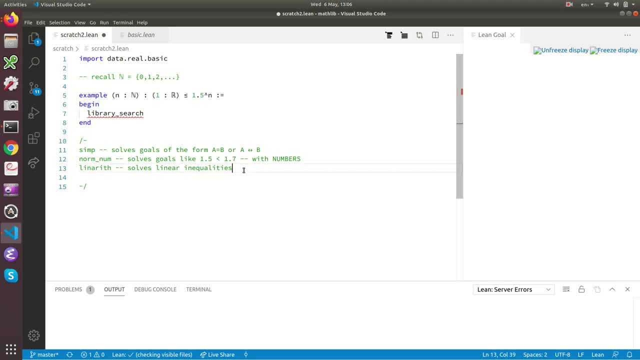 library to try and find this lemma, and library search has failed as well. And why has library search failed? You know looks looks for. you know the exact lemma you need. And the exact lemma we need is that one is less than or equal to 1.5 to the n. 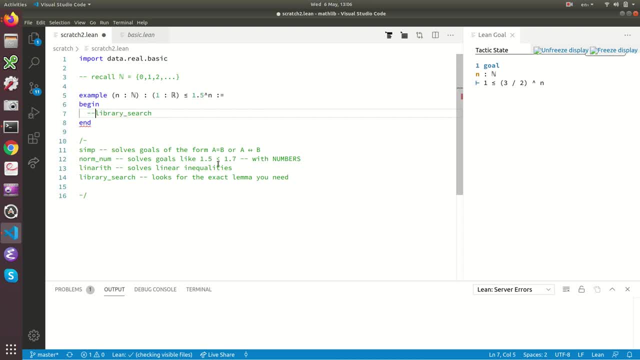 It's not a lemma that's going to be in Lean's maths library, because there won't be any lemmas in Lean's maths library about the number 1.5. this is some other problem. So what the question is, let's step back and say what lemmas will be in Lean's maths library. So 1 less than or equal to. 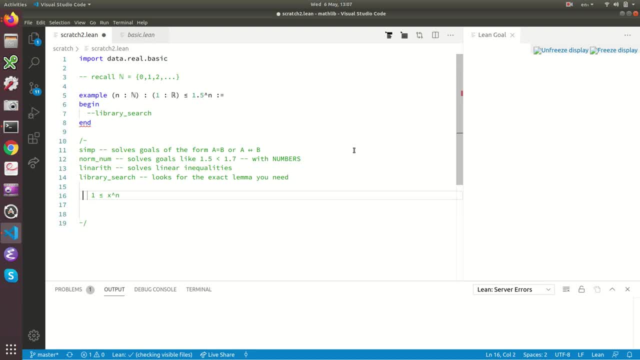 x to the n. that's the kind of result that we need. but you see, this isn't true in general. if x is, for example, a number between 0 and 1, then 1 won't be less than or equal to x to the n. So clearly. 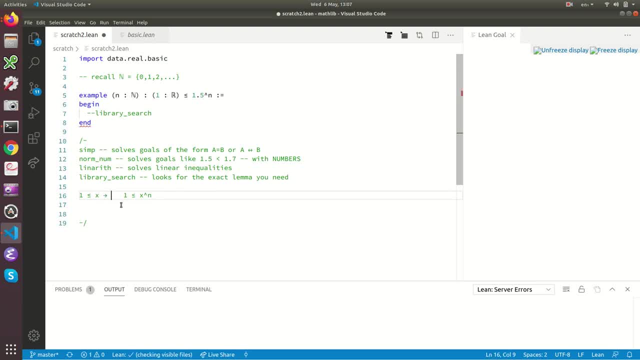 the lemma is this: 1 less than or equal to x implies 1 less than or equal to x to the n. That's the kind of lemma that will be in Lean's maths library. Unfortunately, library search won't find it because the input hypothesis 1 less than or equal to x. I guess in our case that's 1 less. 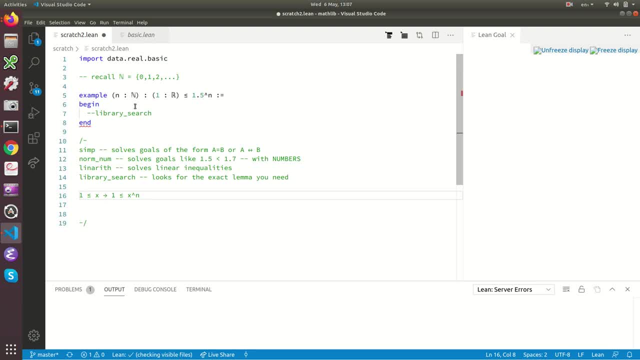 than or equal to 1.5, and 1 less than or equal to 1.5 is certainly provable by Lean, but Lean doesn't sort of know it. Lean has to be told it. So why don't we tell it? have h, the real number 1. 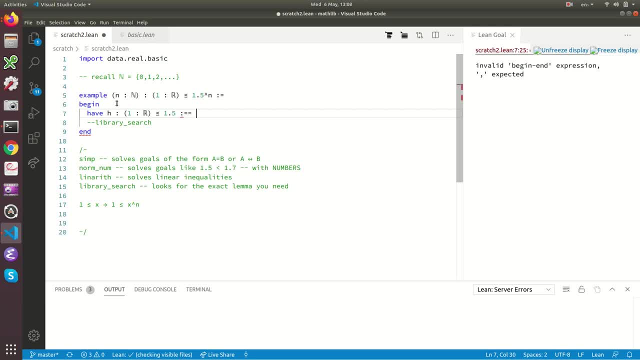 is less than or equal to 1.5. uh, how are we going to solve this, I guess? well, this is: this is an inequality between two explicit numbers, so norm: none will solve this there, and now we're not. we're in a situation where library search might work, so let's try commenting it out. 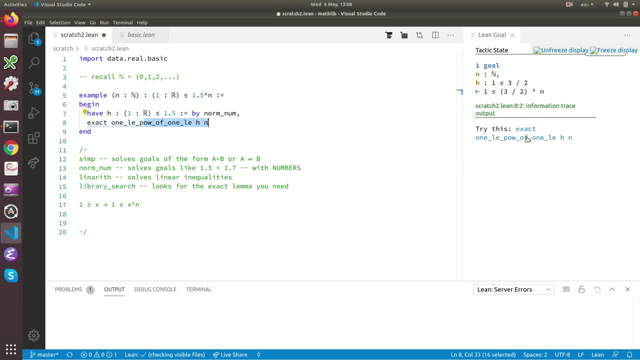 and now we see library search does work. it says: try this, let's click on there. and now we're trying this and this goal has now been solved. You know I put a comma here. we'll see goals accomplished. See, there's no warnings and no errors down here. 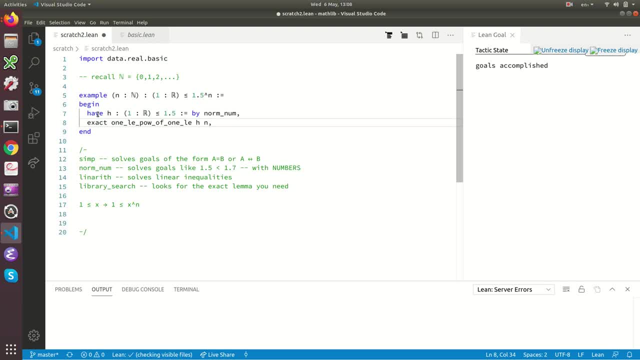 And library search has managed to solve this goal. But you see, we needed this key input here. So when you think about the kind of things that should be in Lean's maths library, it's results like this And lo and behold the moment you put in the hypothesis we need library search will solve it. 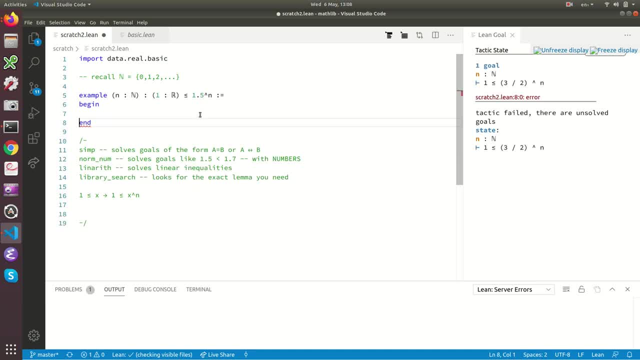 So that's one way of solving lemmas like this. Let me show you another way. The other way involves guessing what the lemma is called. The big problem is, there's hundreds of lemmas. Let's go back to this. Let's go back to this here. 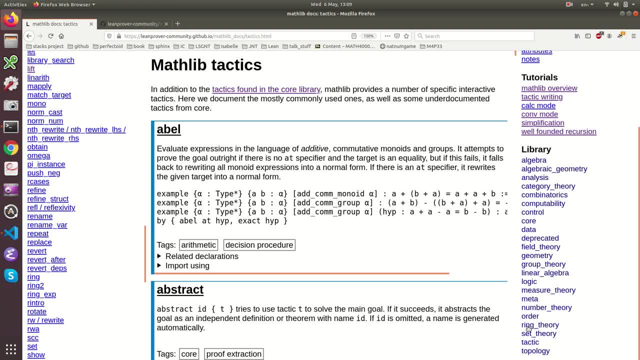 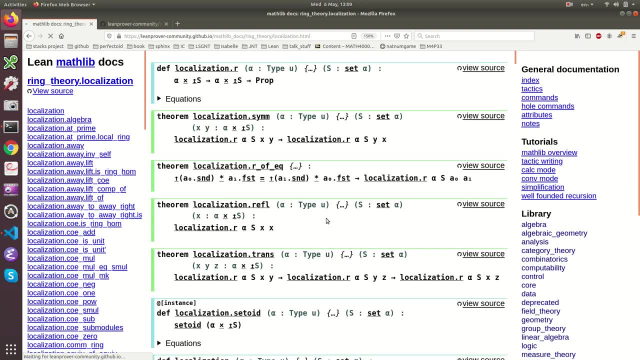 We have like thousands. of you know what's this going to be some lemma about? I don't know. Is it going to be a lemma about ring theory? We click on ring theory and we have a million lemmas about localization of rings. 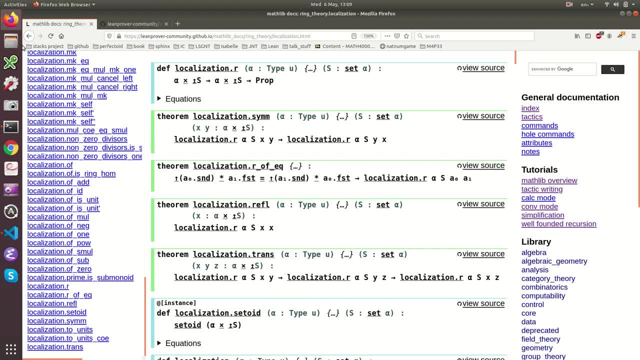 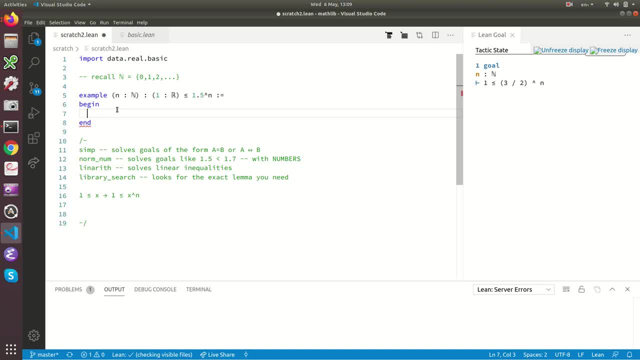 The Lean's maths library has become massive now And if you don't know what you're looking for it'd be quite hard to find the result you're after. But you see there are. These lemmas have all got names and there's some logic behind the names to the lemmas.